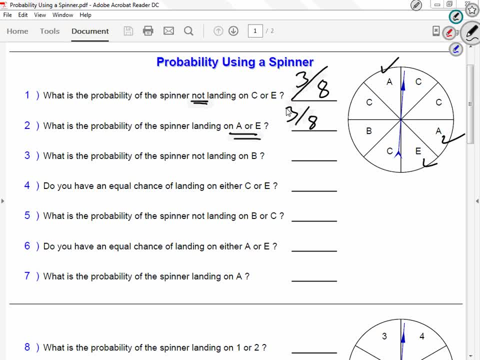 by coincidence, my answer was the same of both, but it's not all the way through. i say it was just coincidence. this probability, it's something. actually we see a lot. um, because i can this fraction, i can make it into a percent, right? three divided by eight gives me a decimal. my decimal can. 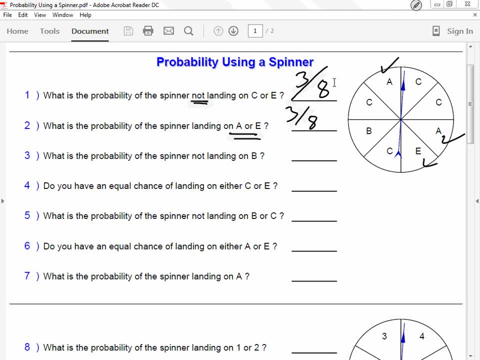 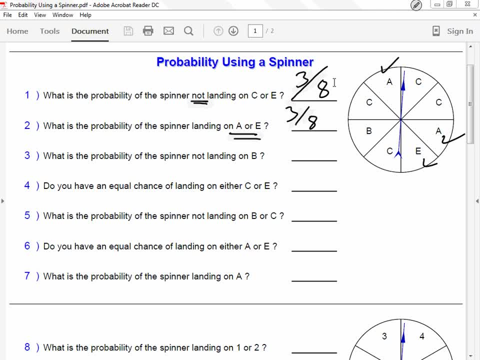 know. so if you guys watch the news and they tell you, uh, probability that a rain is 10, that means it's not going to rain. if you guys watch the news and like, oh, probability to rain is 80, that means it will rain because it's close to hundreds. if they say 40 or 60, that's close to 50. that means. 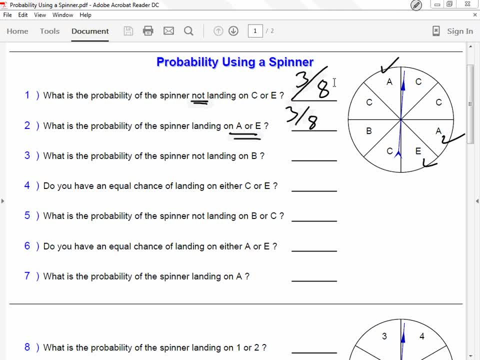 they don't know. so if you, when you ask them, if they tell you probability to rain tomorrow's 40, that means that person does not know. that's basically what they're telling you. i don't know. so, like i said, probability is something we see, but, um, we're looking at it. 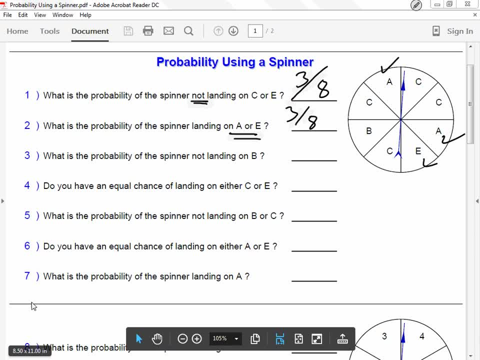 today in fractions, my first seven questions. you guys see my big line in the middle, my set. my first seven questions are relating to the one figure. i have the big line in the middle because that questions 8 through 14 are related to the other thing. but remember, probability is how many can. 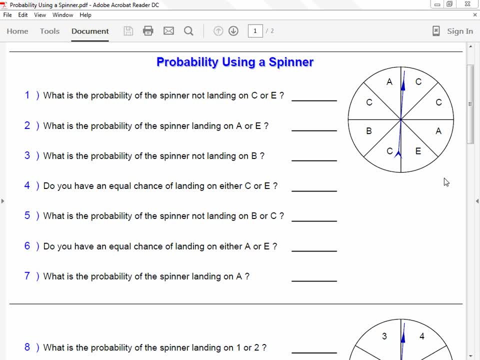 you get over how many they're taught. that's all it is. any questions of probability? number three: i'm looking at number three. what is the probability of the spinner not landing on b? there's a not on b, so i'm going to see how many are not b's? seven out of eight, all right. any other questions?